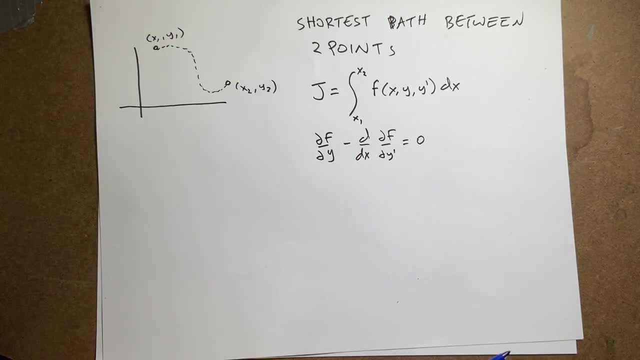 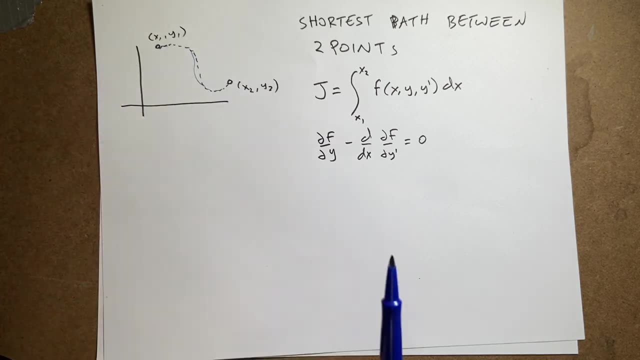 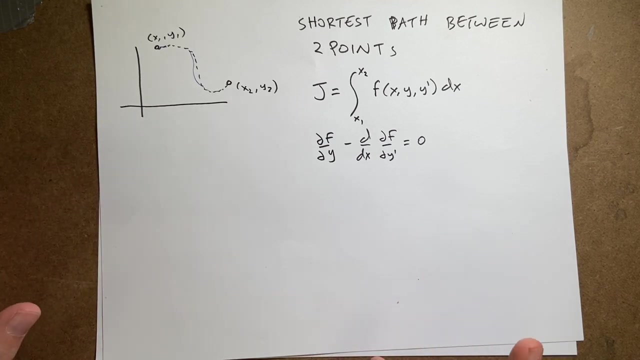 a path. And this is the thing. It's a variational problem. We're not trying to vary one value, We're trying to vary a function, We're trying to vary the function, that is this line. So that makes it much more complicated, And this is our first step into the calculus of variations. So, in general, 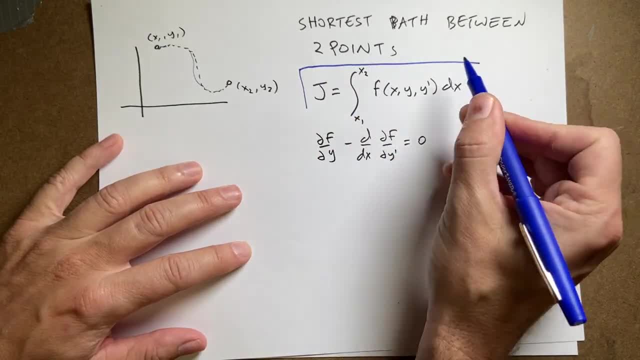 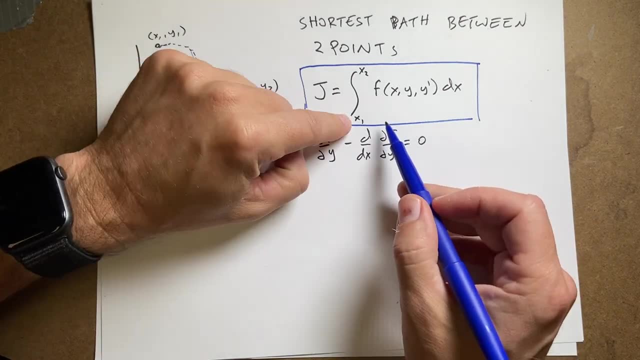 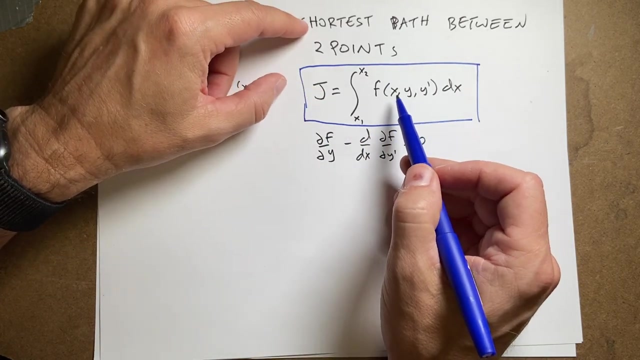 we have this. If I have some integral like this, so j could be anything, I'm just calling it j because i don't know. j is kind of cool and i have some function and i want to minimize, i want to find the function that minimizes the integral. i don't want to minimize the function, i want to find this. 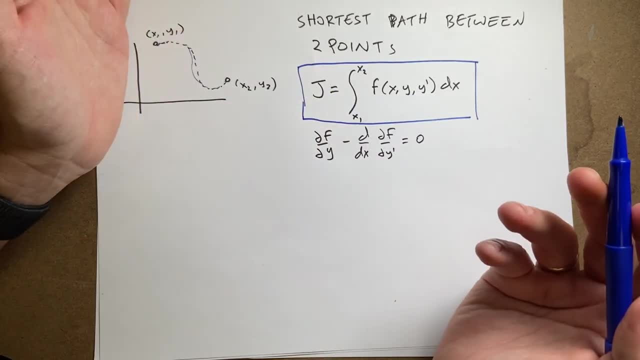 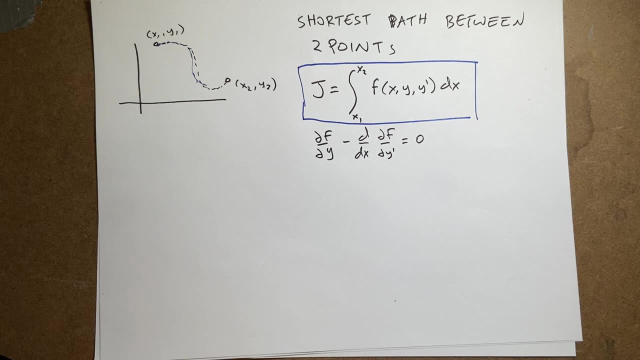 function such that this integral is minimized. and that's what we're doing here, right, because i want to integrate along this path and find the distance, and i want to find what function minimizes that integration. it turns out that the solution is not trivial, but super, super, super useful and very 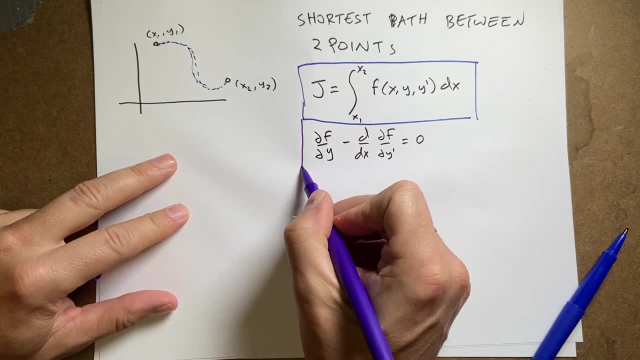 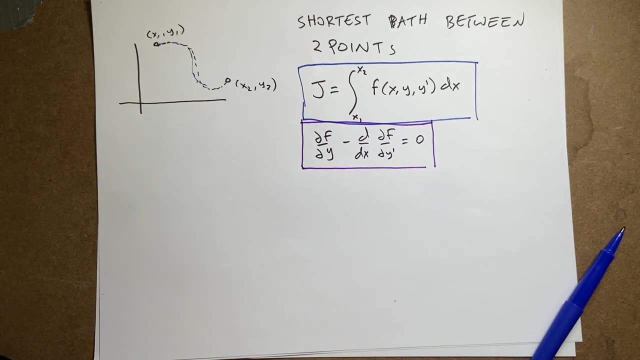 important and it's so useful. i'm going to do it in purple. uh, this is the euler lagrange equation. i'm not going to drive it, okay, but we need to use this to solve this problem, and it turns out that we can use this for a whole bunch of mechanics problems. so this says that if i have a function, 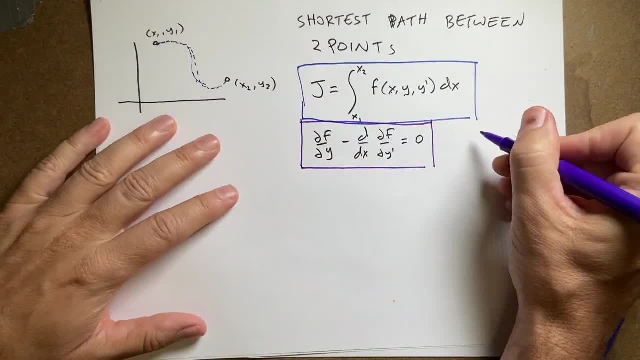 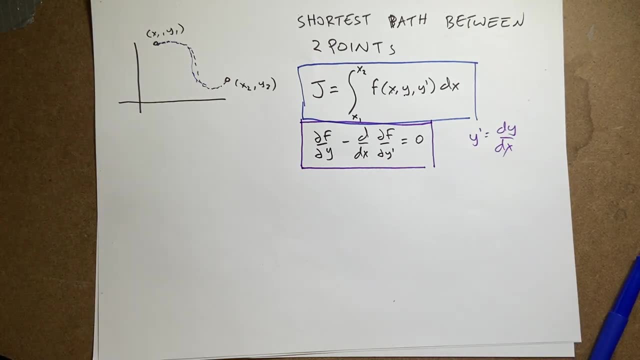 of x, y and y prime. and y prime, just to be clear: y prime is dy, dx, i mean, and i'm using the variables x and y, but we could use uh, x and t, or you know whatever. it doesn't matter, and that's what's great about. 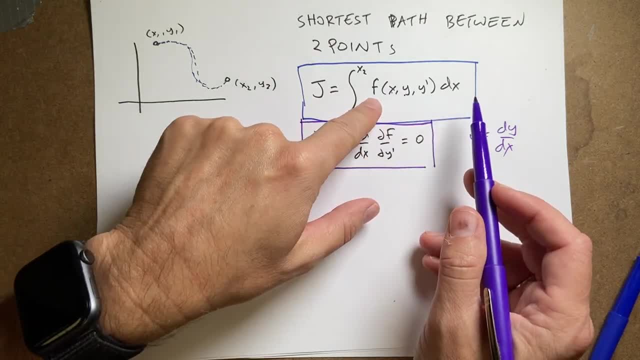 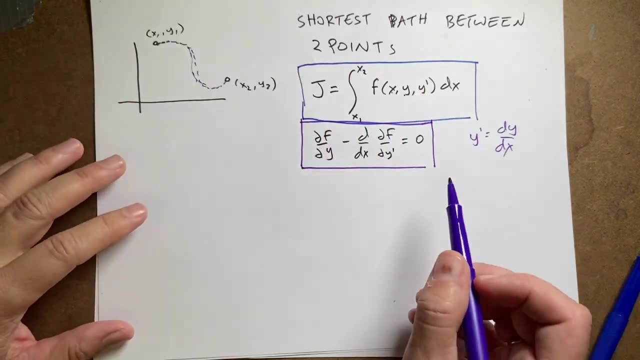 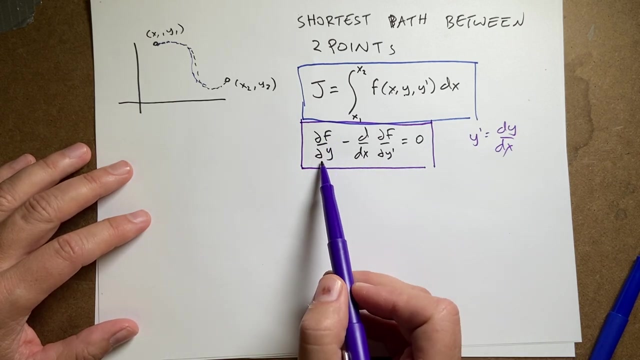 this doesn't matter what your variables are, but i need: uh. this integral depends on the x function, the y, the value of x, it could be y and the derivative of y. then the function that minimizes this has to satisfy this equation. that says the partial of f with respect to y, minus the derivative. 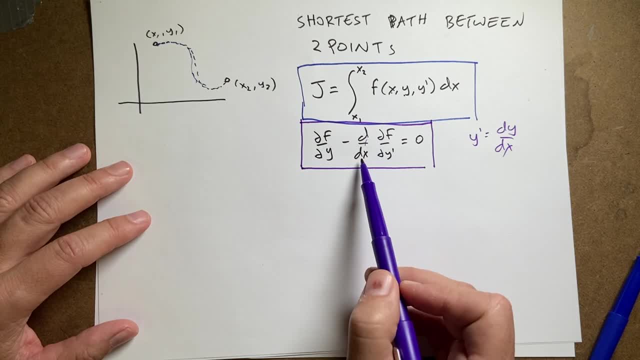 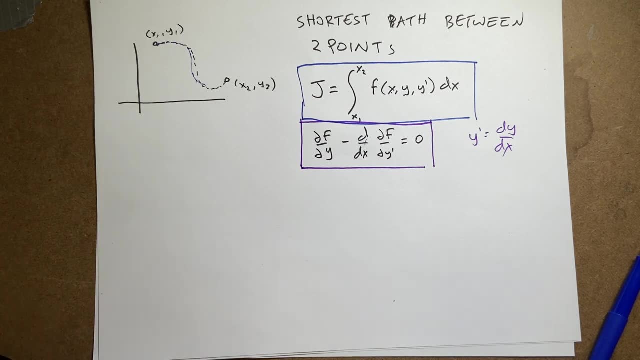 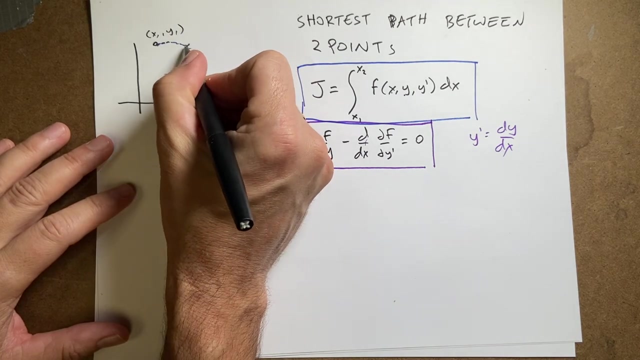 remember, these are partials, not derivatives. and that's an actual derivative. the derivative with respect to x of the partial of f with respect to y, prime is equal to zero. so let's do it. how do you do this? to show that the path between two points is a straight line. so let's pick a little piece, right? 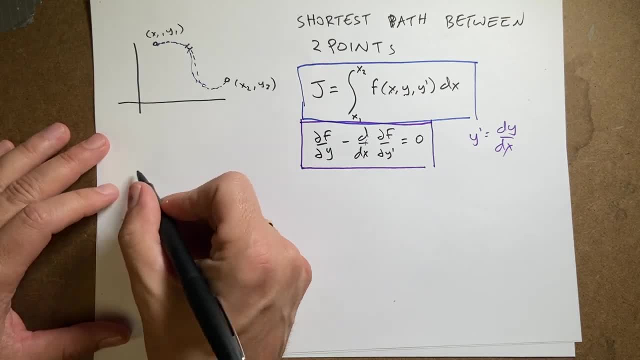 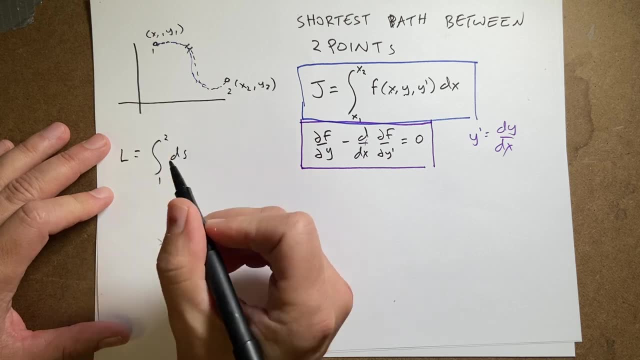 here. what i'm going to do is say, uh, what's the path link? i'm going to say l equals the integral from. i'm just going to call this one to two. one to two of ds, where ds is the sum of the little pieces along that function. 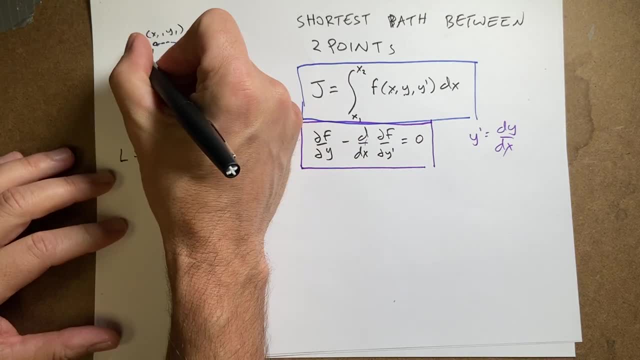 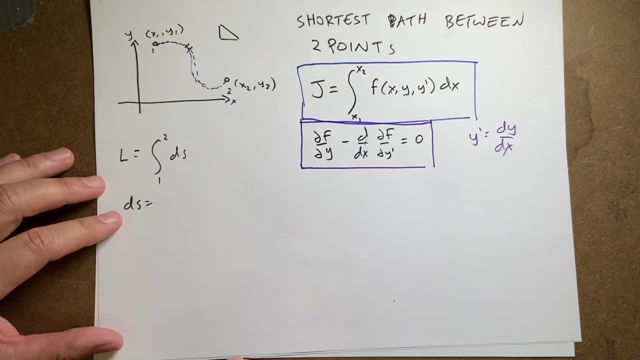 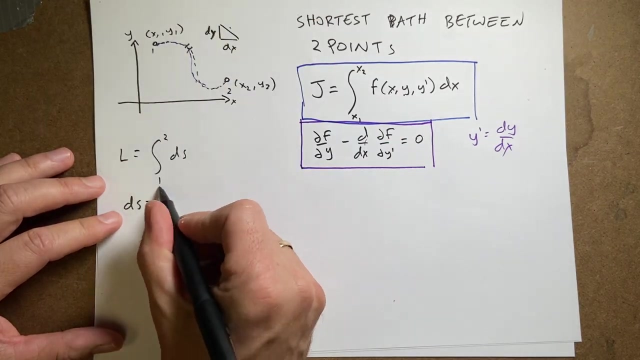 so in cartesian coordinates x, y, in two dimensions, then ds is going to be. you can imagine this. right? there's my little path piece. this is dx, that's dy, that's a y. so that would be the hypotenuse, so it'd be the square root of dx squared plus dy squared, and that's my function i'm going to put in. 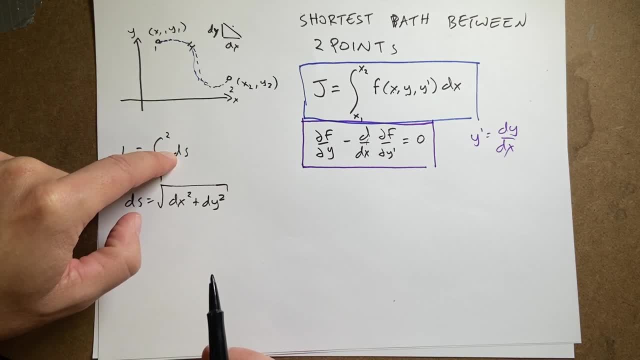 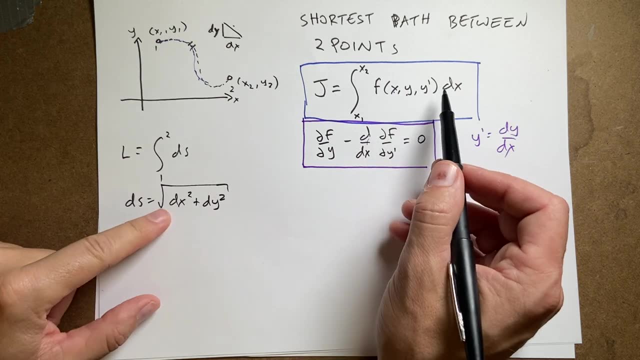 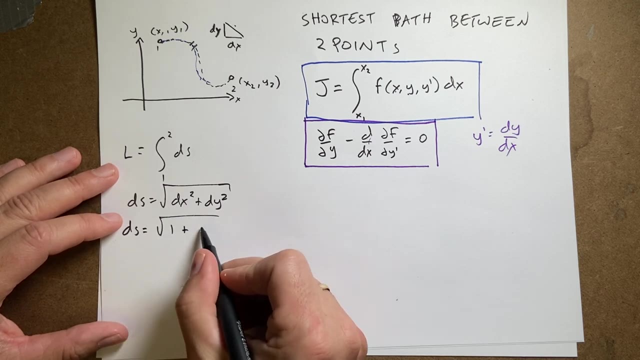 there, but i can't do that right because, um, i don't, i don't have it in this form. i have a dx, i have a dy, i just want dx. so let's write this as a ds equals the square root of one, plus d, y, d, y. 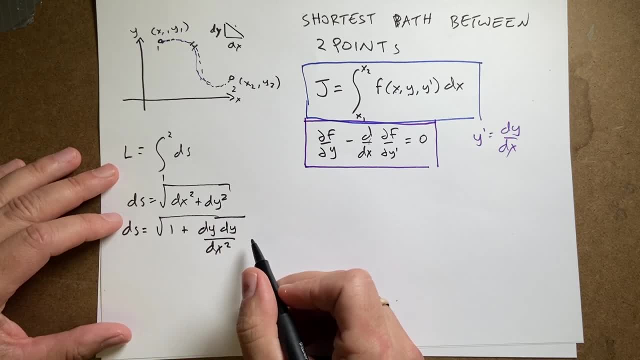 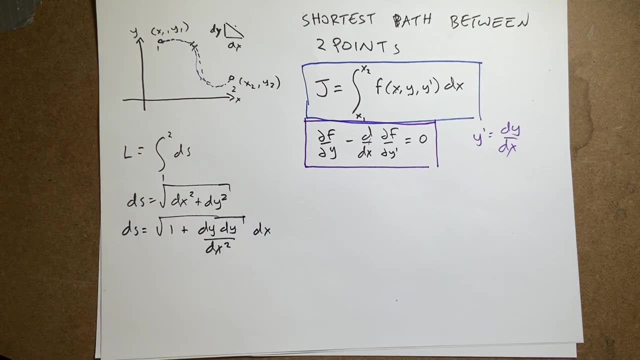 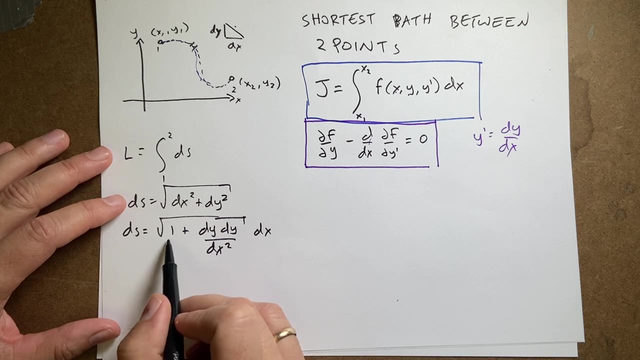 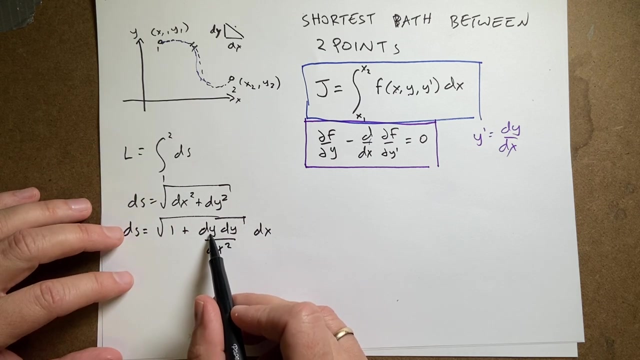 dx squared. well, i don't know what i'm doing here, dx. i had a trick, so i have to factor it out. the dx right, because this is um. i divide everything by dx squared. yeah, that's right. so then i have um. i want to say this is: uh, yeah, yeah, yeah, that's going to be, this is dy. 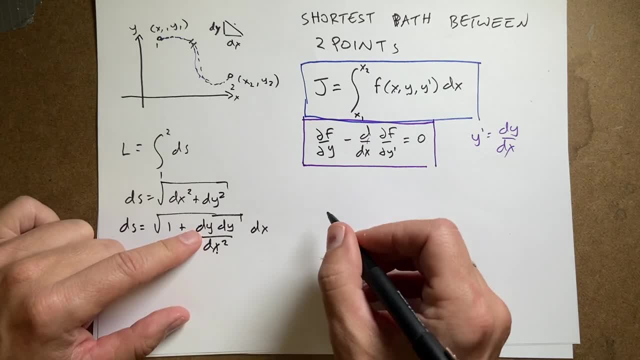 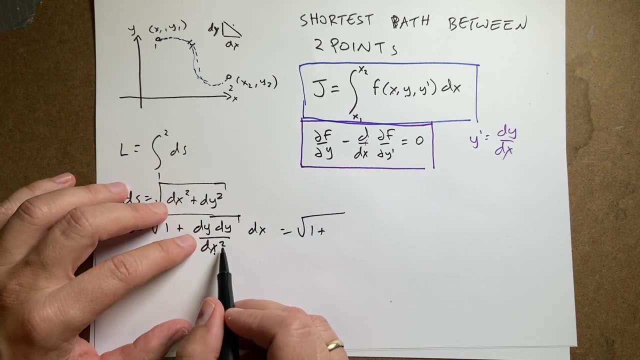 dx squared. right, i should have left it that way. so it's d. it's equal to the square root of one, plus this is going to be dy dx- quantity squared. it's not the second derivative, it's the quantity squared, So this is actually y prime squared. 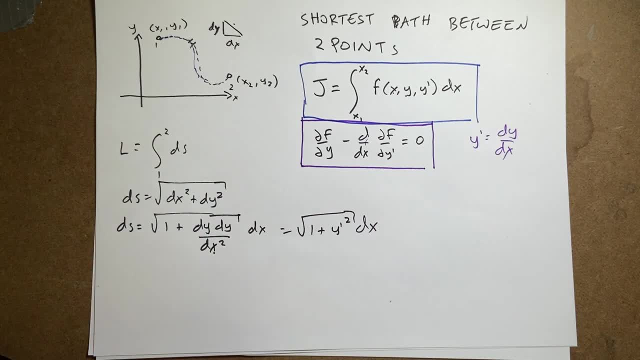 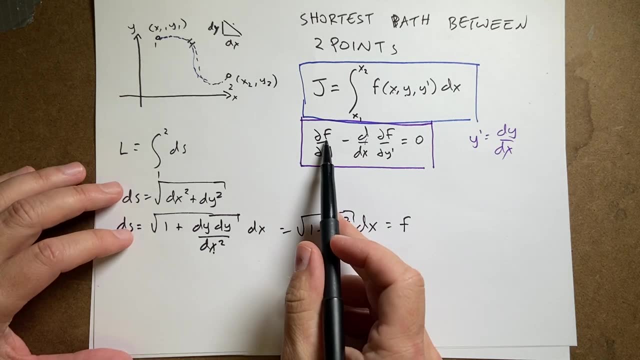 Now I don't have the dy in there, right? I don't have to worry about that. I have it in this form. So that's my f, So I can now do my partial derivative. So the first thing I'm going to do is take the partial derivative of this with respect to f. 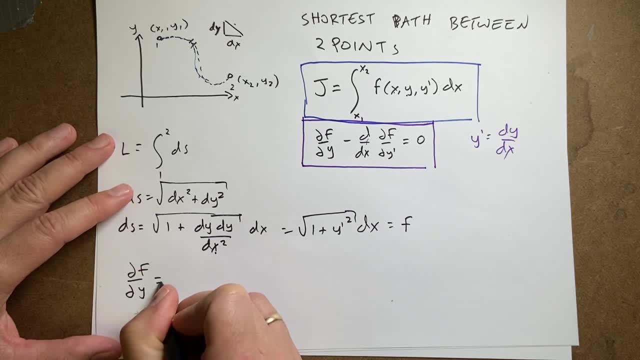 I mean y. That's pretty easy. The partial of f with respect to y is equal to 0.. Why? Well, there's no y in there, right, And it's a partial derivative, so it doesn't really matter. That's easy. 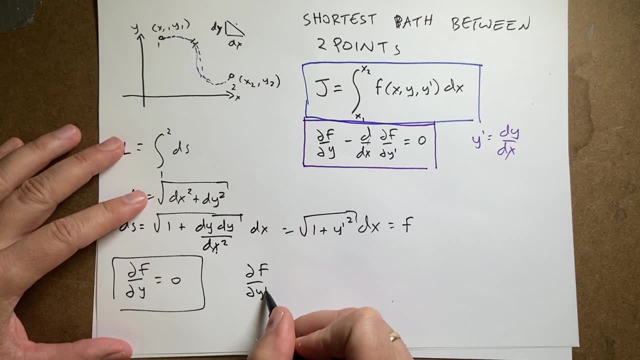 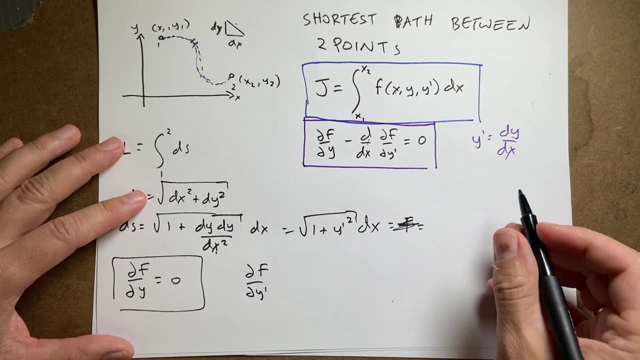 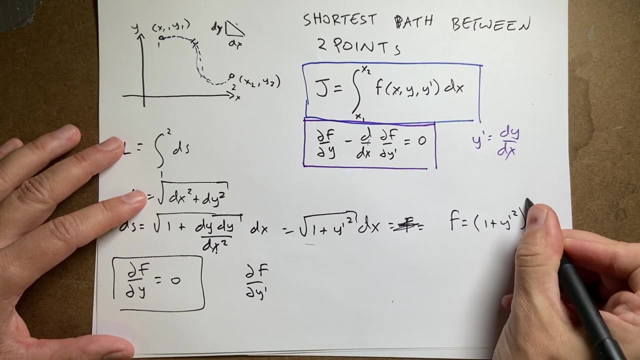 Now I can take the partial of f with respect to y prime, So I'm going to write this as actually this is not f. f is just the square root part, So I'm going to write it as 1 plus y prime squared to the 1 half. 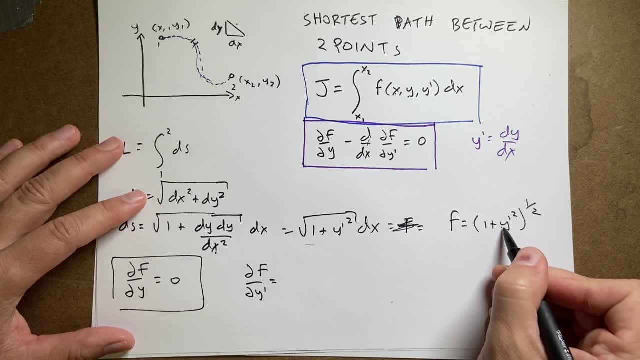 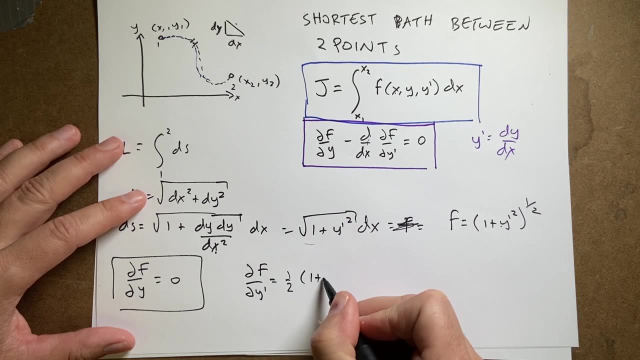 because I like to think of things that way. So if I take the partial of that with respect to y prime, I can use the chain rule. It's going to be the derivative of this, which is 1 half times 1, plus y prime squared to the negative 1 half right. 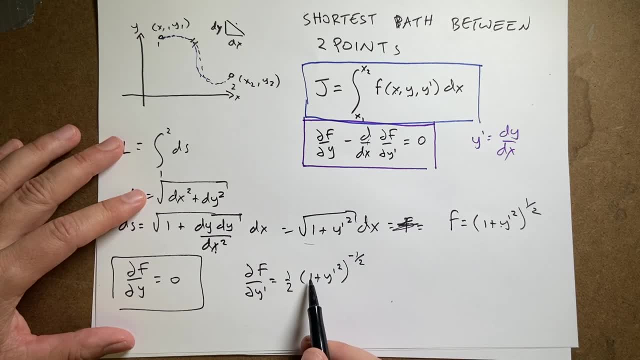 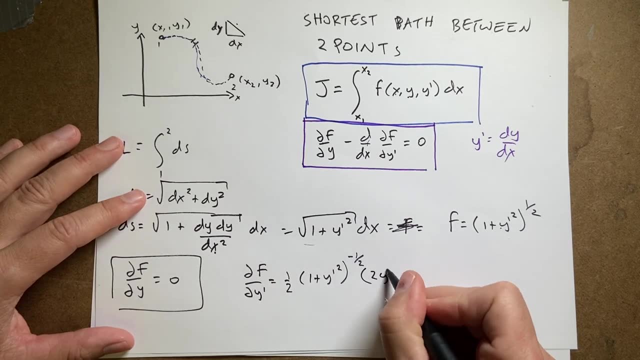 I have to decrease that by a power of 1.. Now I have to take the derivative of the stuff inside. The derivative of 1 is 0.. The derivative of y, the partial with y prime squared, is going to be 2y prime. 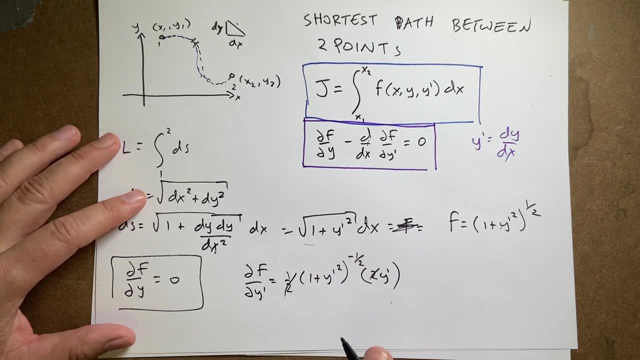 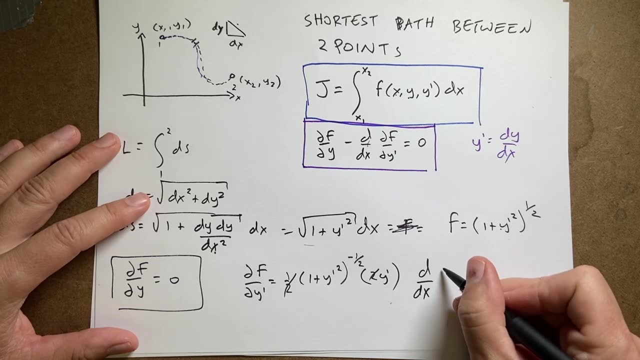 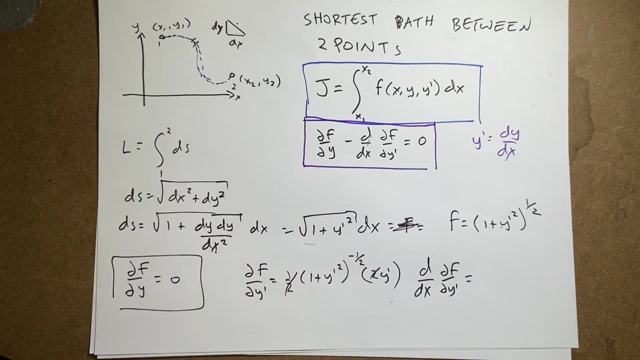 And the 2s cancel. So now I need to find d, dx, why I could, of the partial of f with respect to y prime. I could do that right And I would have to take the derivative of all these terms, but I'm not going to. 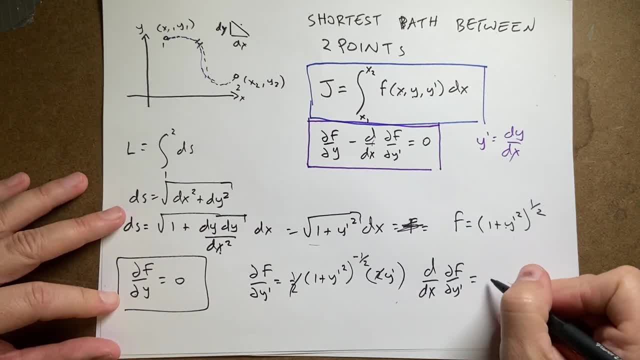 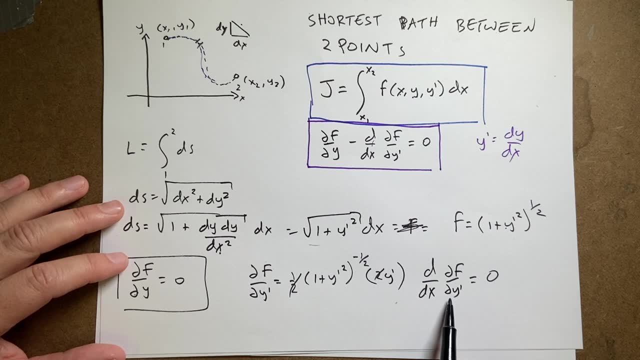 Because I know this is. since this is 0,, this is 0. The derivative of f prime f with respect to y prime is 0, which means the partial of f with respect to y prime is a constant right. If I take the derivative and I get 0, then this part right here has to be a constant. 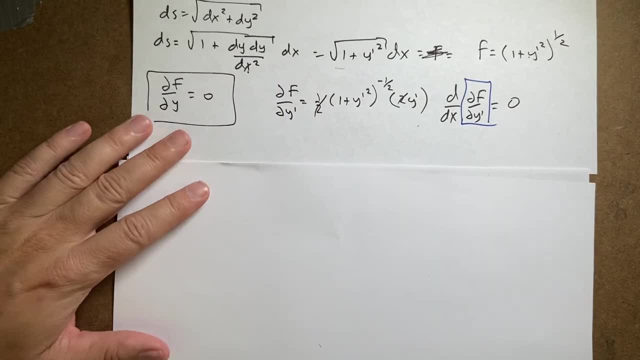 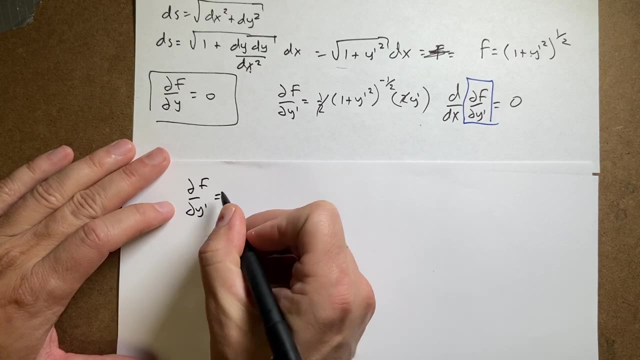 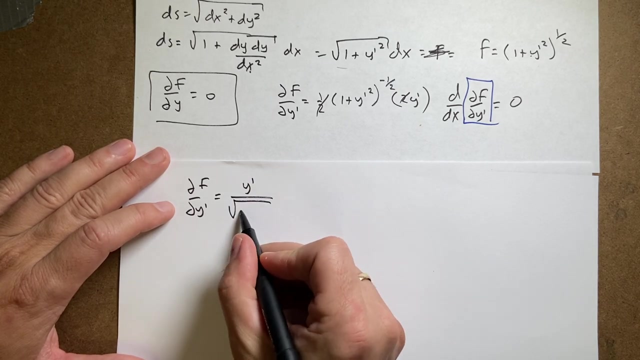 Okay, so let me Move to my next page and I will say this. I hear my function partial of f with respect to y prime. it's going to be this stuff. I'm going to write it as: y prime divided by the square root of 1 plus y prime squared equals c. 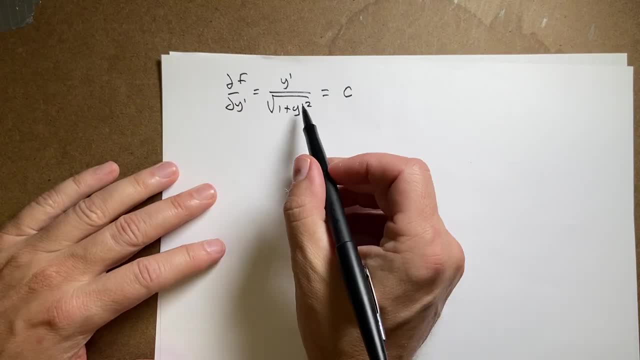 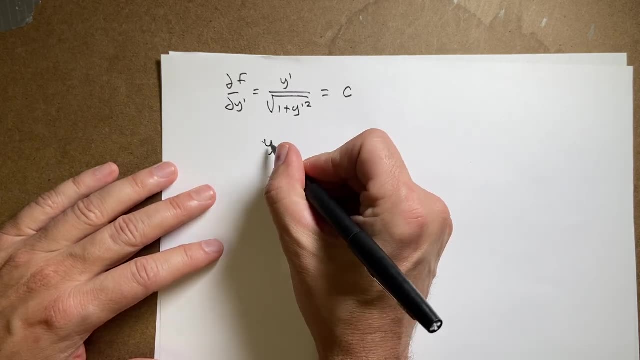 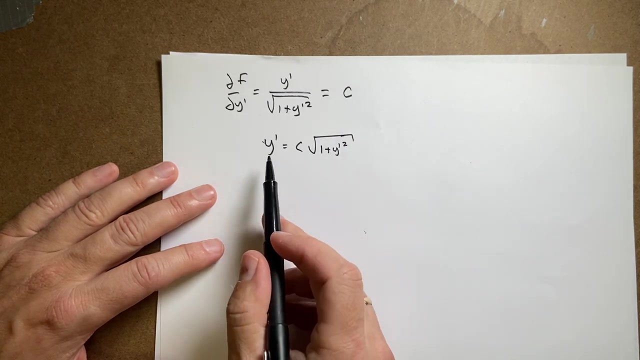 Some constant. So let's just multiply both sides by this to get rid of the fraction, And I get y prime equals c, the square root of 1, plus y prime squared. Now I'm going to square both sides and I get y prime squared equals c squared. 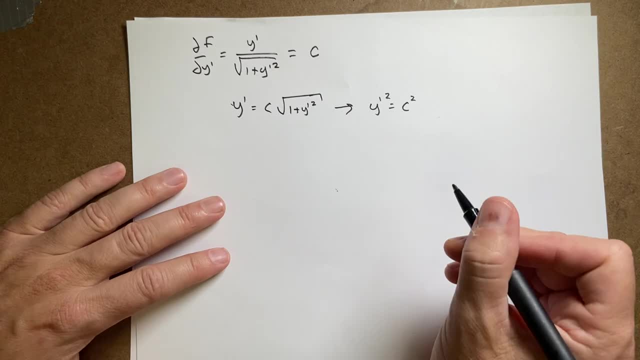 But I mean you can just call it c if you want. A lot of people do that. I'm going to. I'm not going to do that. I'm going to write it as c squared because I care about you guys. 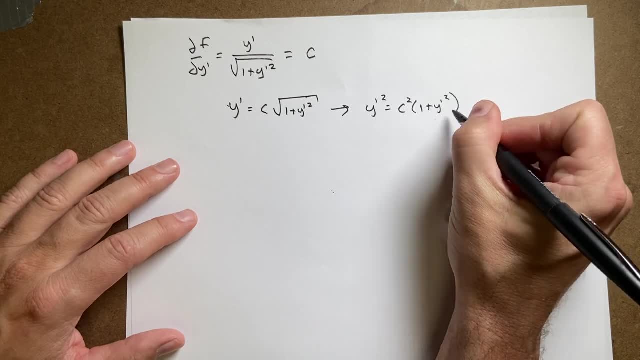 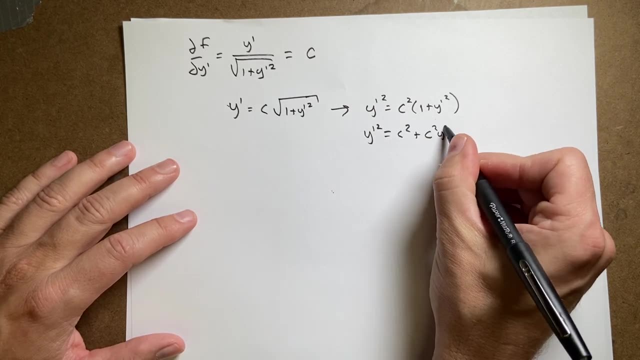 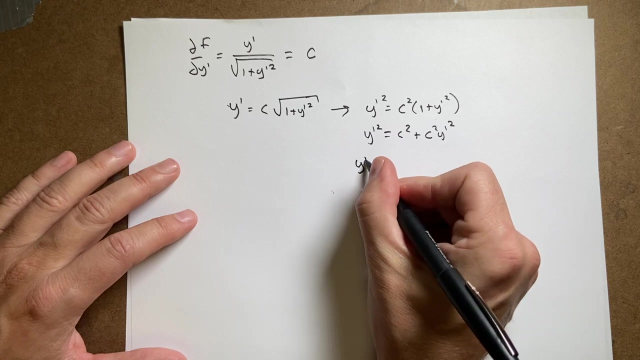 Times 1 plus y prime squared. Now let's multiply this out and I get y prime squared equals c squared Plus c squared y prime squared. Now I'm going to subtract this from both sides. It doesn't really matter. I'm going to say y prime squared minus c squared, y prime squared. 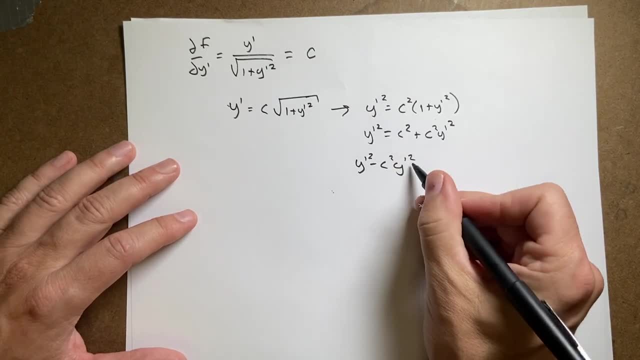 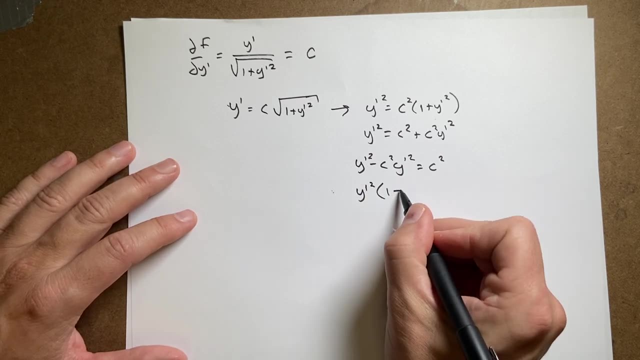 And I'm doing way more work than I need to. You could just you could stop earlier. But equals c squared, And then I'm going to factor out the y prime And I get y prime squared times. 1 minus c squared equals c squared. 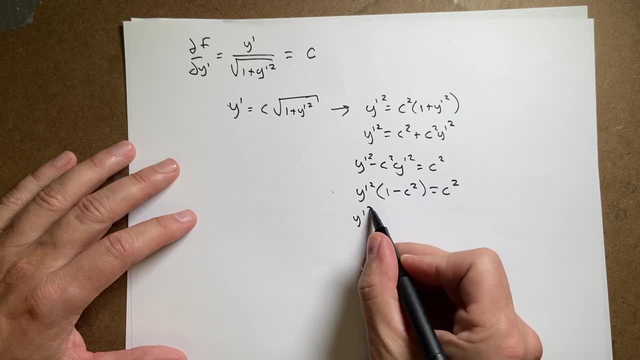 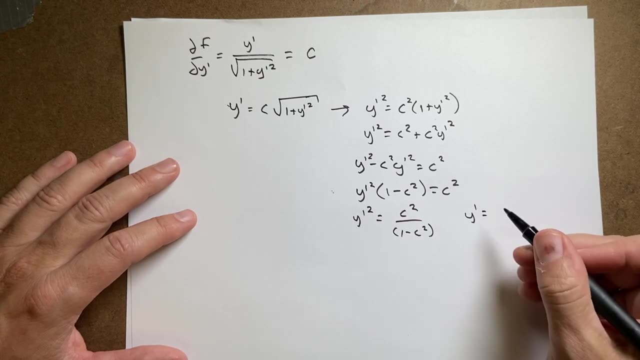 And now I get y. now I'm going to divide both sides by this: Y prime squared Equals c squared over 1 minus c squared. And then I take the square root: Y prime equals a constant. I'm going to call it k. 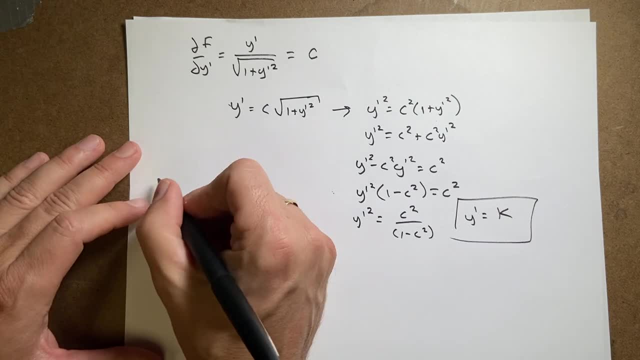 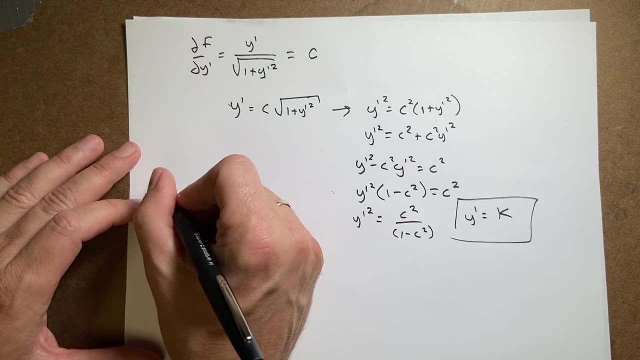 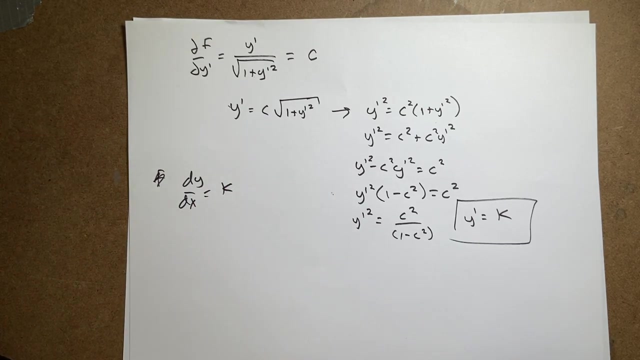 So this is my solution, right there. I want a function f such that the slope is constant. That's what that says. This says: dy: dx equals some constant. Well then, what's y and what's x? Well now I'm actually done. 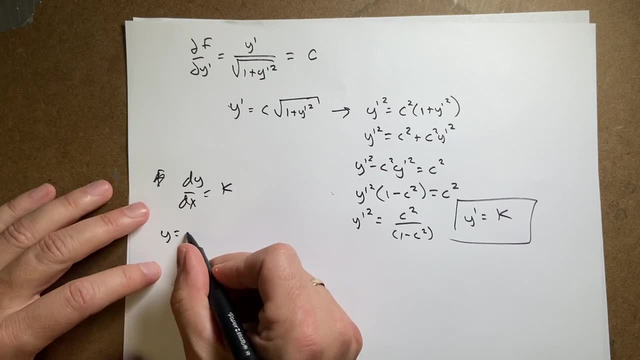 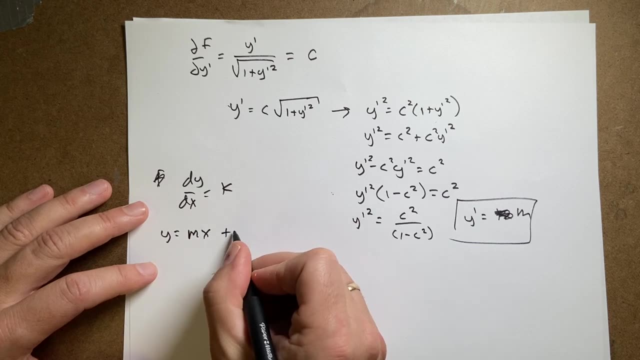 Because if the, if the slope is constant, I can use this: Y equals some constant. I'll call it now m. Actually, I should have called that m, That would have been funny. m x plus b, Right, And I can get that by integrating both sides. 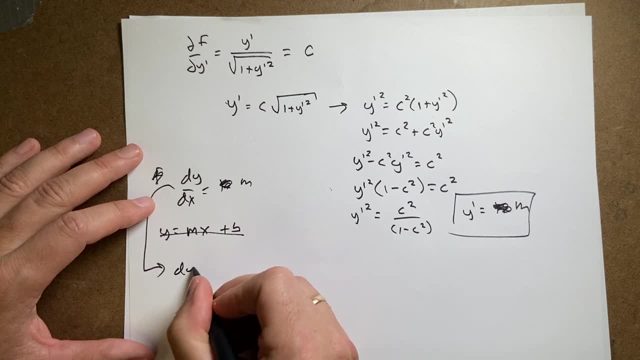 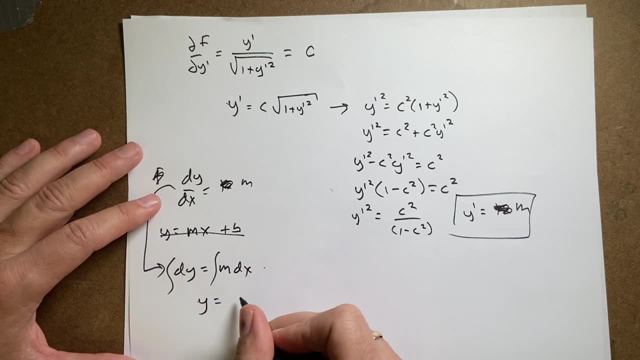 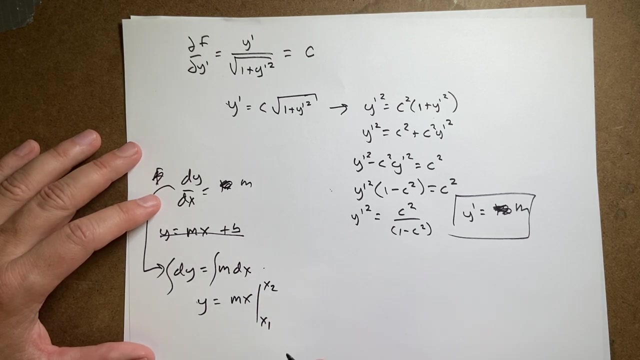 I can actually just do that. So let's say dy equals m, dx, I integrate both sides and I get y equals m, x From x1 to x2.. So it's going to be m And this is from y1 to y2.. 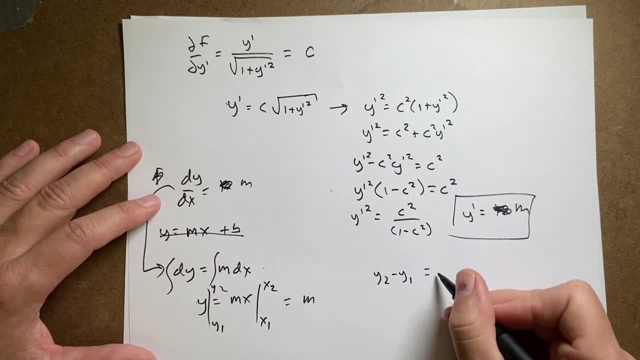 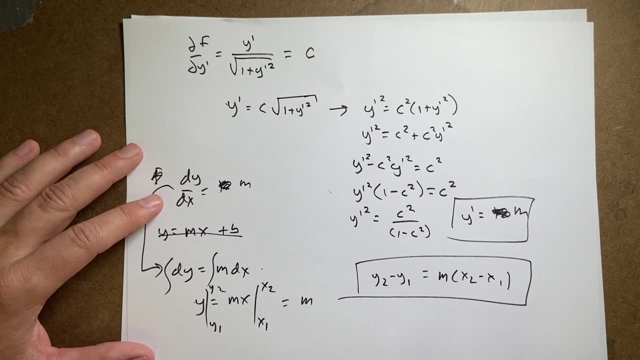 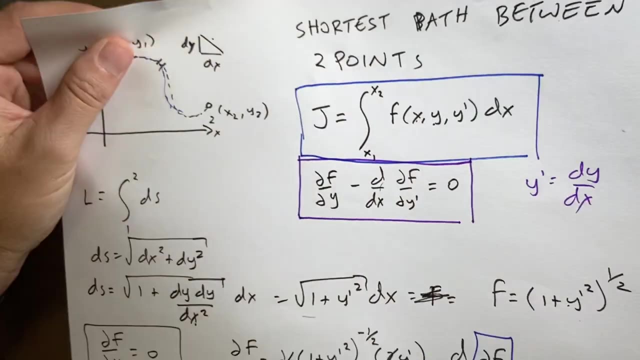 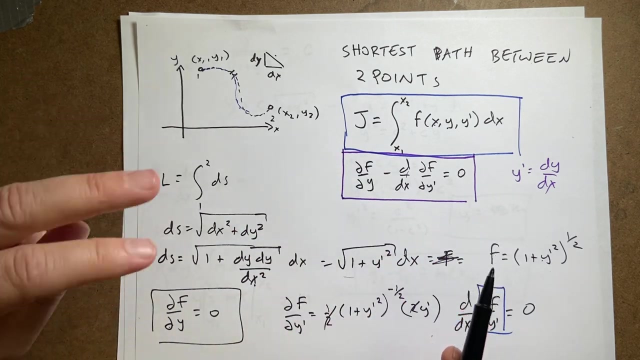 So I get y2 minus y1 equals m, x2 minus x1.. And that's my function, Which is a line, The end. So I mean, I think it's Confusing sometimes to see this, Because you kind of have to do two things that I don't really like. 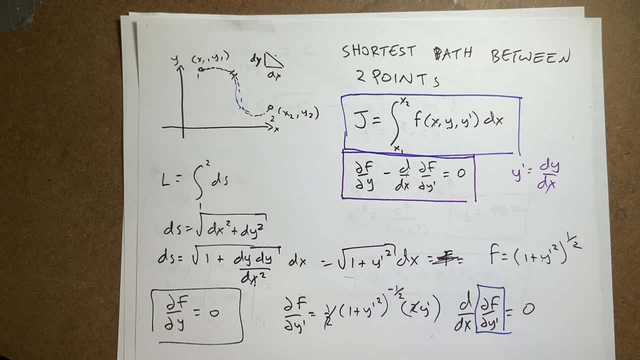 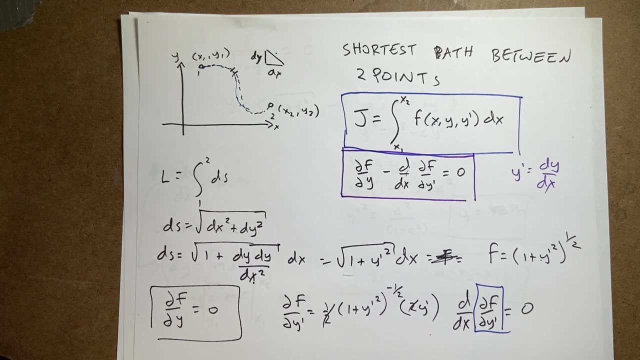 One use this Euler-Lagrange formula. What I didn't show where that came from. It's kind of I don't really want to derive it right now. And number two is this: getting this y prime squared, This y prime, and they're getting rid of the dy.